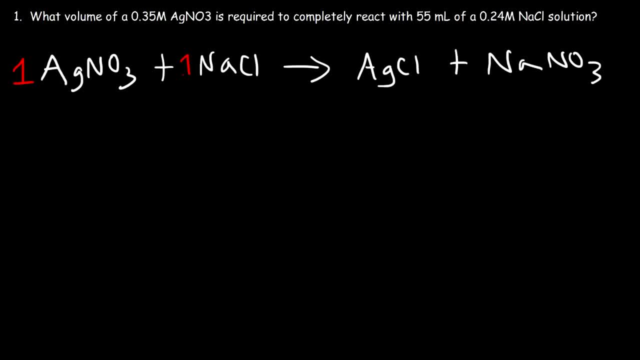 So the chemical equation is already balanced. Now, how can we use this information to find the volume of silver nitrate? If you want to find the volume of silver nitrate, start with the other substance, sodium chloride. Now keep in mind molarity. 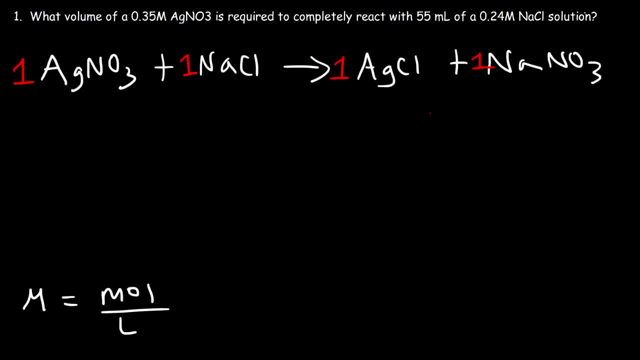 can be represented by the volume of silver nitrate. It can be represented as moles per liter, which is what I'm going to do here. So a 0.24 molar solution means that there's 0.24 moles of sodium chloride. 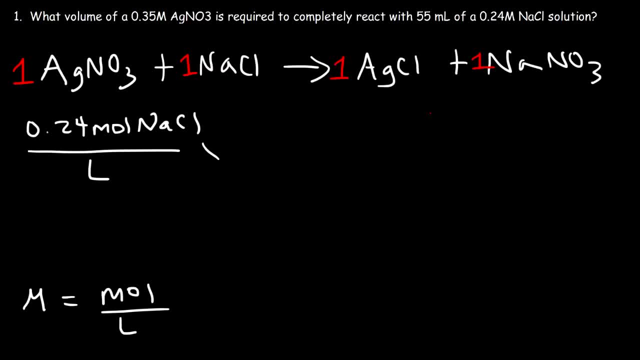 per one liter of solution. Now let's multiply it by the volume. We need to convert 55 milliliters into liters. To do that, simply divide 55 by 1,000.. So that's going to be 0.055 liters. 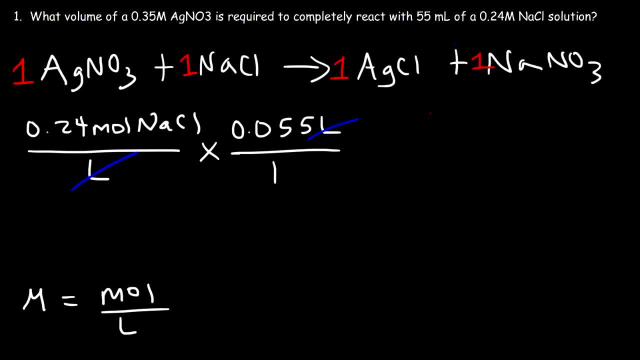 And now we can do the same thing with the other substance. We can cancel the unit liters. Now, the next thing we need to do is change the substance from NaCl to silver nitrate, And we can use the molar ratio to accomplish that. 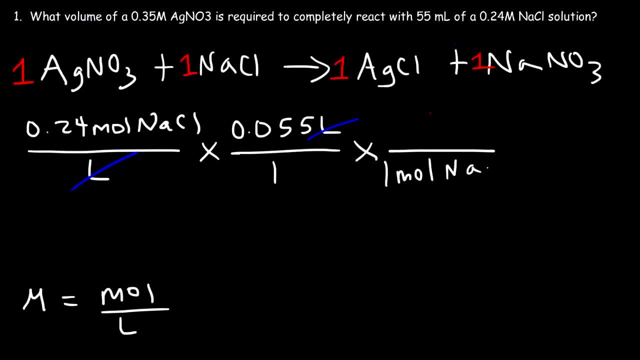 So one mole of NaCl will react with one mole of AgNO3.. Now the next thing we need to do is convert moles to liters. We can do that using the molarity of the silver nitrate solution. So a 0.35 molar solution means that there's 0.35 moles of silver nitrate per one liter of solution. 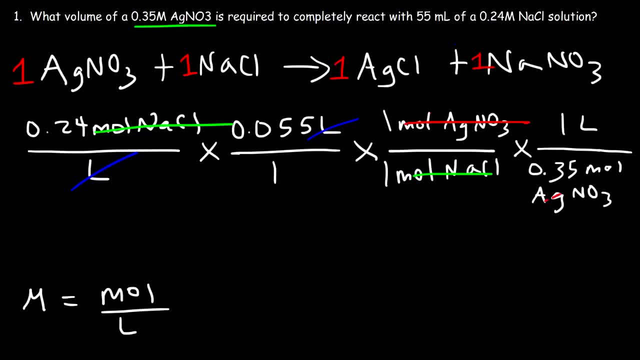 So now we can get rid of these units And now we have the volume in liters. So it's going to be 0.24 times 0.24.. 24 times 0.055 divided by 0.35, and so you should get 0.0377 liters. and if you multiply, 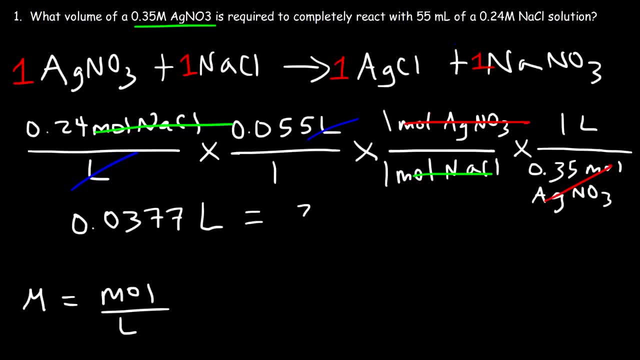 that by 1000, that's equivalent to 37.7 milliliters. So that's the volume of silver nitrate that's required to completely react with that solution. Now there's another equation that you can use to get the same answer. 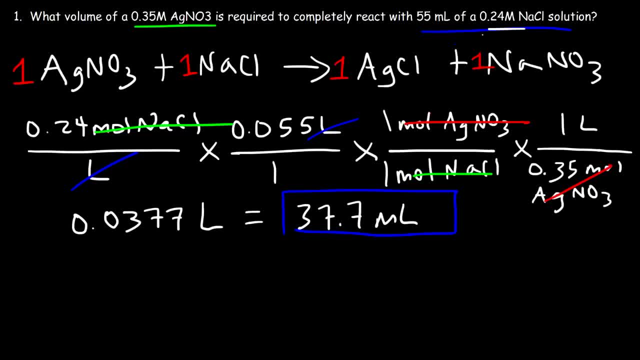 So anytime you see in a problem, molarity volume, molarity volume- you can use this equation: M1V1 is equal to M2V2.. So on the left, I'm going to use M1V1 with reference to silver nitrate and M2V2 I'm going 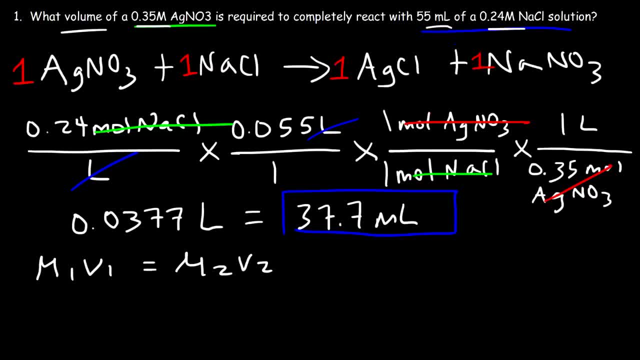 to use it with reference to sodium chloride. So M1 is the concentration of silver nitrate, which is 0.35, we're looking for the volume of AgNO3, M2 is 0.24 and V2 is 55.. 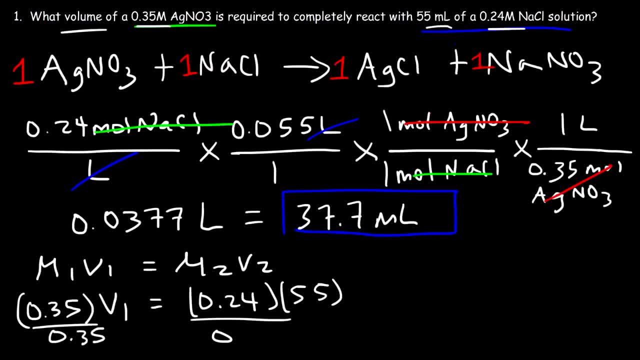 So all we got to do is divide both sides by 0.35.. So V1 is going to be equal to 0.24 times 55 divided by 0.35.. And so this will give you the same answer: 37.7 milliliters. 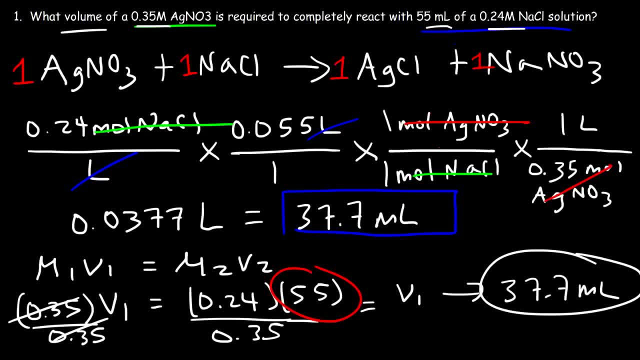 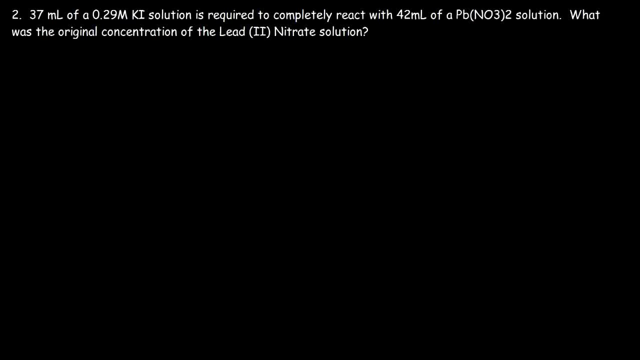 Now it's important to understand that if V2 is in milliliters, V1 is going to be in the same unit, milliliters, as well. Number two: 37 milliliters of a 0.29 molar potassium iodide solution is required to completely. 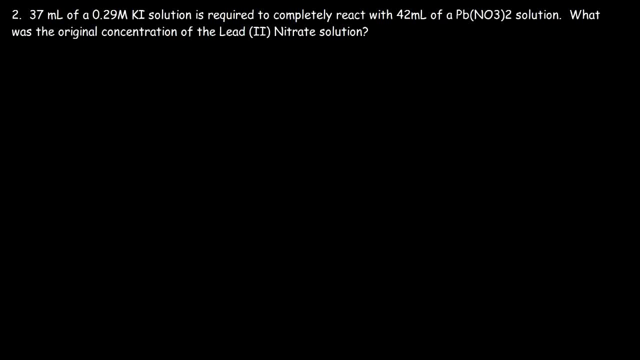 react with 42 milliliters of a lead nitrate solution. What was the original answer? No concentration of the lead nitrate solution. So once again, let's begin with a balanced chemical equation. So lead nitrate reacts with potassium iodide. 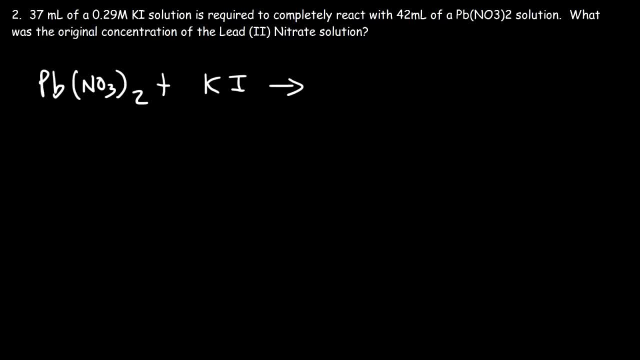 So we have another double replacement reaction. So lead is going to pair up with iodide Now. lead has a positive 2 charge, as indicated by the Roman numeral, and plus the fact that there's two nitrates attached to it, Iodide has a minus 1 charge. 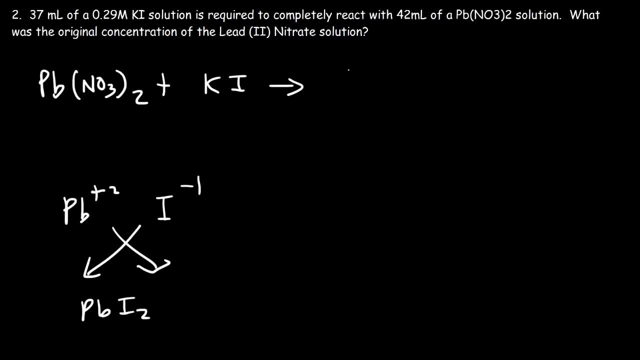 So lead iodide contains the formula PbI2.. Now we need to pair up potassium and nitrate. Potassium has a positive 1 charge, Nitrate has a negative 1 charge. If the magnitude of the charges are the same, you could simply write them together. 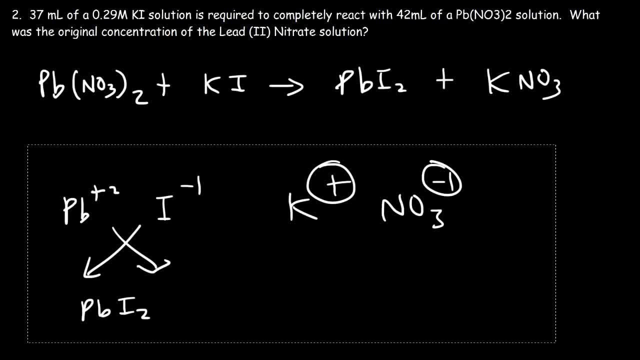 So it's KNO3.. Now our next step is to balance this reaction. Notice that there's two nitrates on the left side, So therefore we've got to put a 2 in front of KNO3.. And we have two iodide ions on the right side, so we've got to put a 2 in front of Ki. 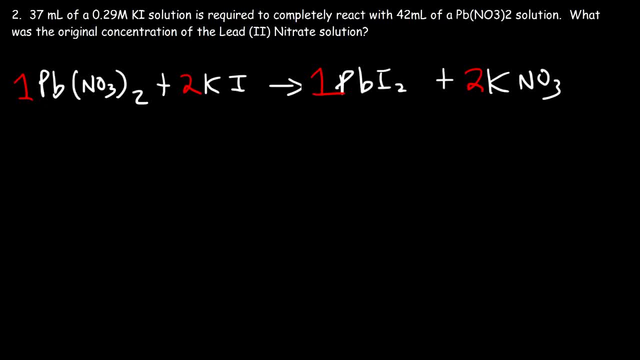 And now the chemical equation is balanced. Now, in order to find the original concentration of lead nitrate, Let's start with the other substance, Ki. Now, whenever you see the word molarity, you could write it as moles per liter. So a 0.29 molar solution means that there's 0.29 moles of Ki per 1 liter of solution. 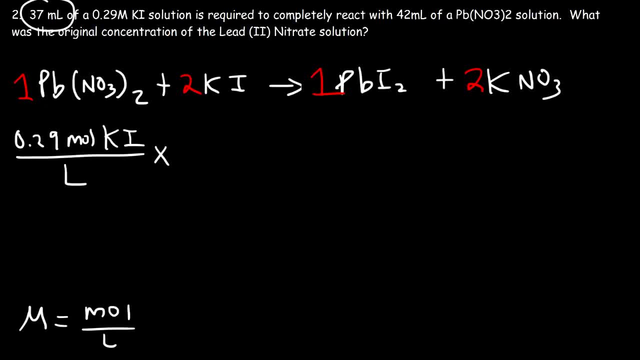 Now what we need to do is multiply by the volume in liters, So to convert 37 milliliters into liters, Multiply by 1,000. So that's going to make it 0.037 liters. So we can cancel the unit liters. 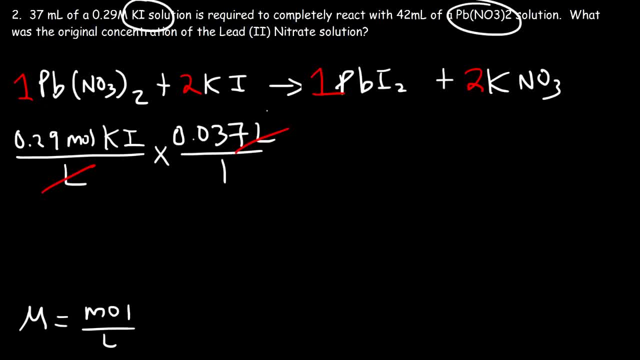 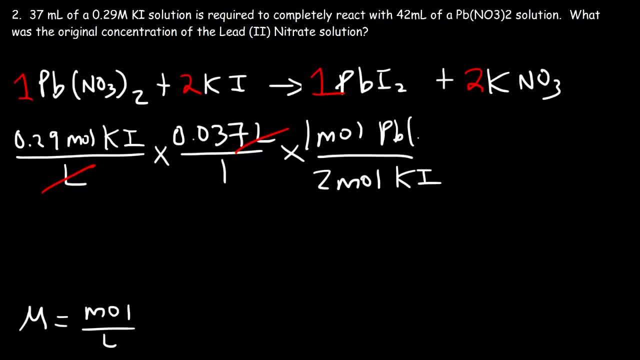 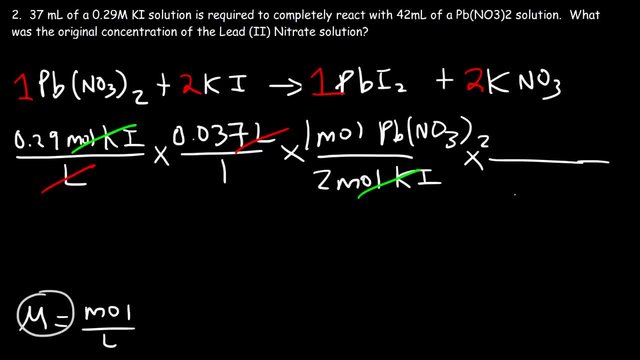 It's 42 milliliters If we divide that by 1,000.. That's 0.042 liters, 1.042 liters. So now we can do the math: It's 0.29 times 0.037 divided by 2, and then divided by 0.042.. 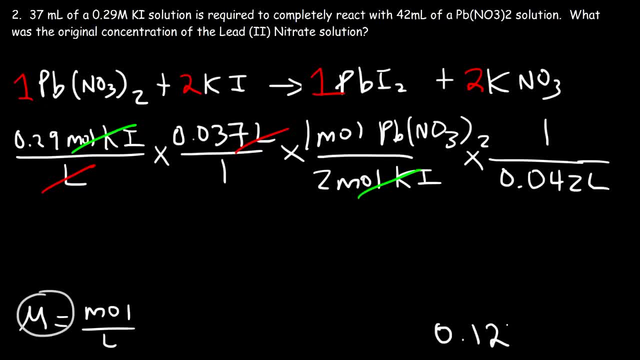 So the concentration is 0.1277 moles per liter of lead nitrate. So let's see if we can get the same answer using the formula M1V1,, which is equal to M2V2.. Now we can get the same answer. 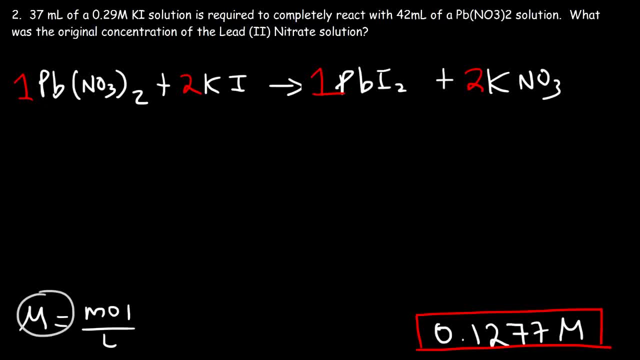 But we just have to be careful in the way in which we use it, Because we need to incorporate the molar ratio in this reaction. M1V1 is going to correspond to this substance. lead 2 nitrate. M2V2 is going to correspond to potassium iodide. 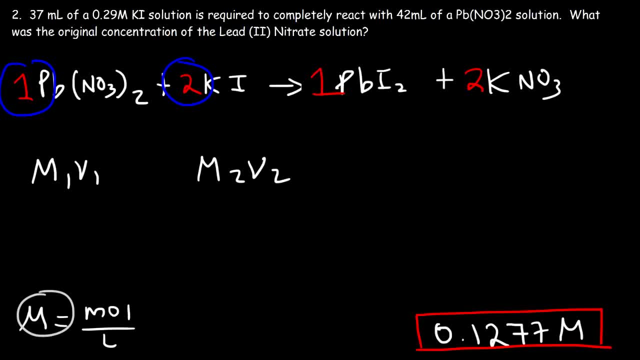 Now what you need to do is you need to exchange the coefficients with coefficients. in this equation, You've got to reverse them, So this one is going to go over here And the 2 is going to go on the other side. If you do it this way, the equation will give you the right answer. 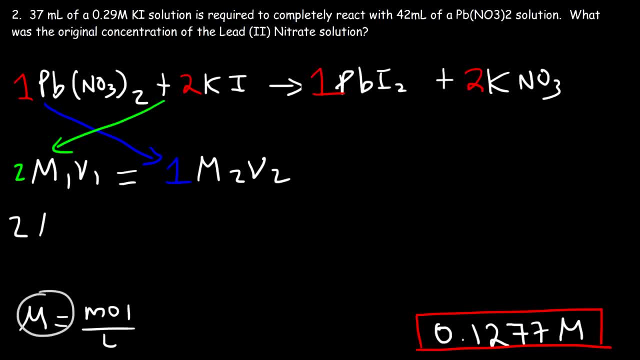 Now, M1 is the molarity of lead 2 nitrate, which is what we're looking for. V1 is the volume of lead 2 nitrate. That's 42 milliliters. M2 is 0.29.. And V2 is 37.. 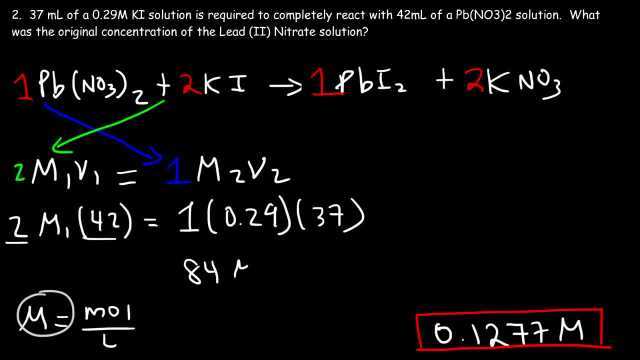 So let's multiply 2 by 4.. That's 42,, so that's 84.. And then 0.29 times 37,, that's 10.73.. Now, in order to get M by itself, we've got to divide both sides by 84.. 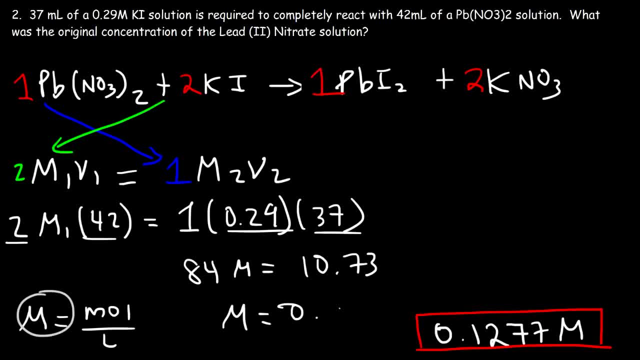 10.73 divided by 84, that's 0.1277.. So, as you can see, we get the same answer. So any time you have a problem that has molarity, volume or something like that, you're going. 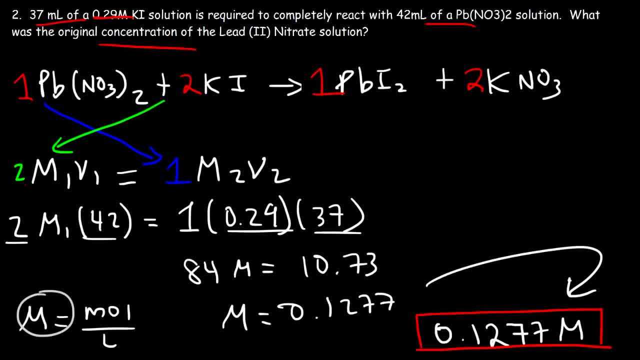 to use this equation: Molarity and volume. You can use this equation, but you need to write a balanced chemical equation. You need to find out what the molar ratio is and incorporate it into the equation. If you do that, then you can use the equation to get the right answer. 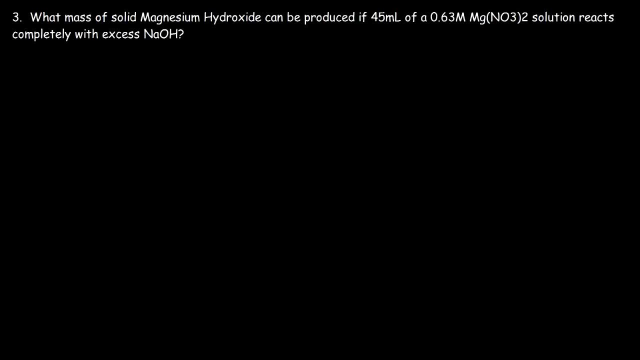 Number 3.. What mass of solid magnesium hydroxide can be produced if 45 milliliters of a 0.63 molar magnesium nitrate solution reacts completely with excess sodium hydroxide? Now we can't use the formula M1V1 equals M2V2 because we're not looking for molarity or 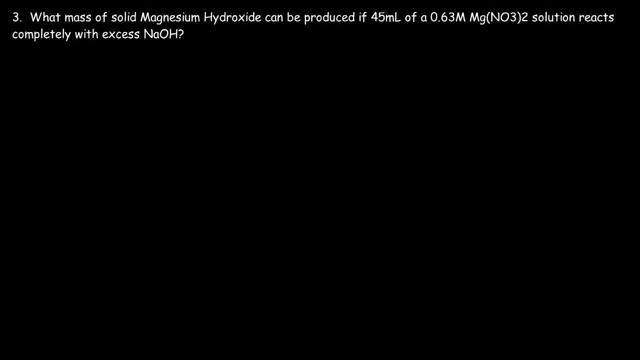 volume. We're looking for the mass. Let's write a balanced chemical equation first. So we know that magnesium nitrate is reacting with sodium hydroxide. Magnesium is going to pair up with hydroxide 4M. Magnesium has a plus 2 charge. 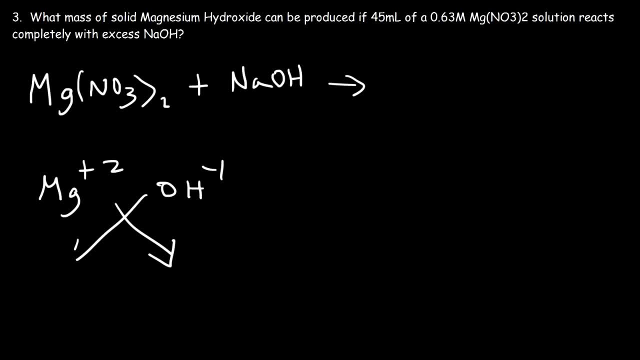 Hydroxide has a minus 1 charge, So to combine them, it's going to be Mg1OH2.. Whenever you have multiple polyatomic ions in a compound, you need to enclose it using parentheses. So this is MgOH2.. 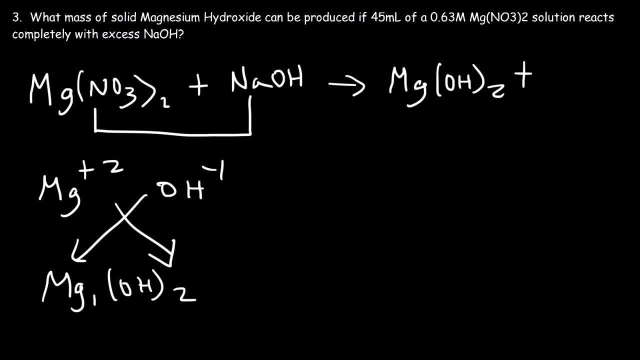 Now the other product comes from pairing Na and NO3. They both have the same mass, They have the same magnitude of charge, So we can write them in a 1 to 1 ratio. Now let's balance the chemical equation. So we have two nitrate ions on the left. 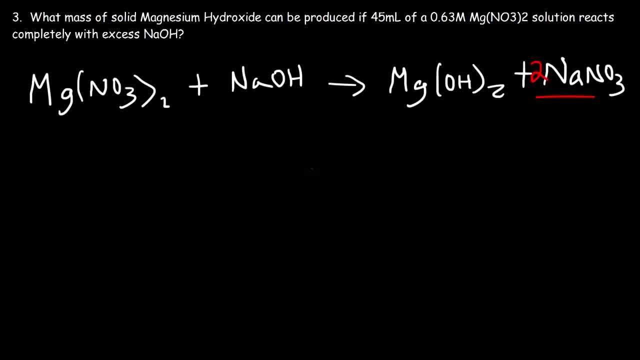 Therefore we need a 2 in front of NaNO3.. So now we have two sodium ions on the right, So we need a 2 in front of NaOH, And now everything is balanced. So our goal is to find the mass of sodium hydroxide. 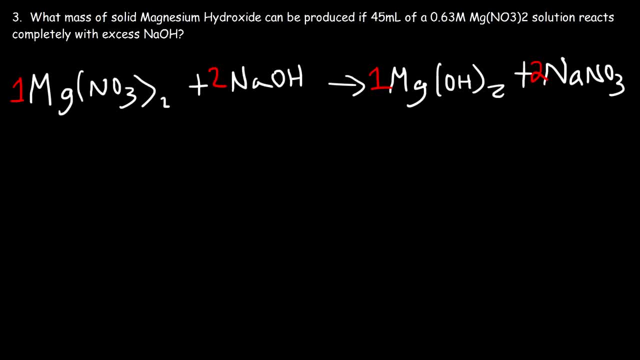 So we're going to do that. The mass in grams of magnesium hydroxide- Now, sodium hydroxide is the excess reactant. Magnesium nitrate is the limiting reactant, So therefore we can base our calculations on the quantity of magnesium nitrate. 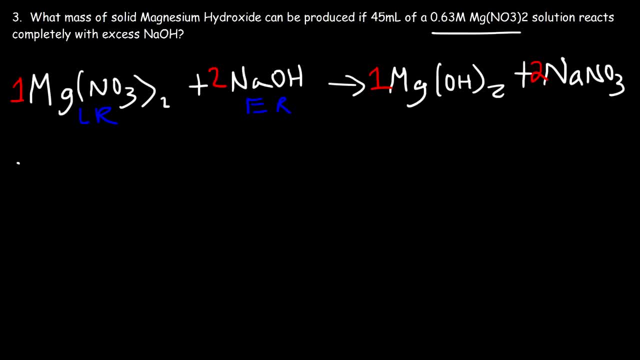 So let's start with the molarity of magnesium nitrate. So it's 0.63 moles of MgNO3O2 per liter of solution. So that's 0.63 moles of MgNO3O2 per liter of solution. 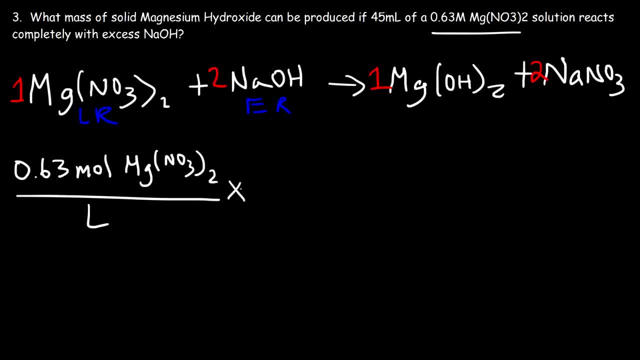 So that's 0.63 moles of MgNO3O2 per liter of solution, And now let's multiply it by the volume in liters, though. So if you divide 45 by 1,000, it's going to be 0.045 liters. 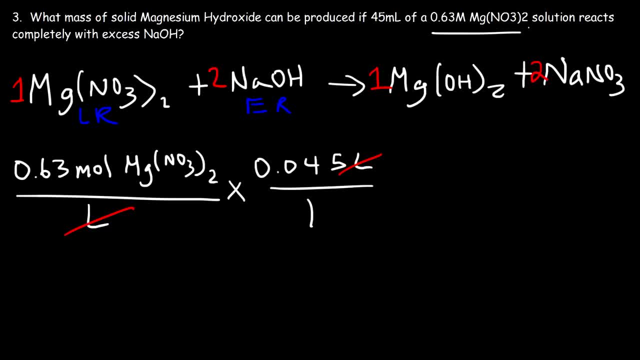 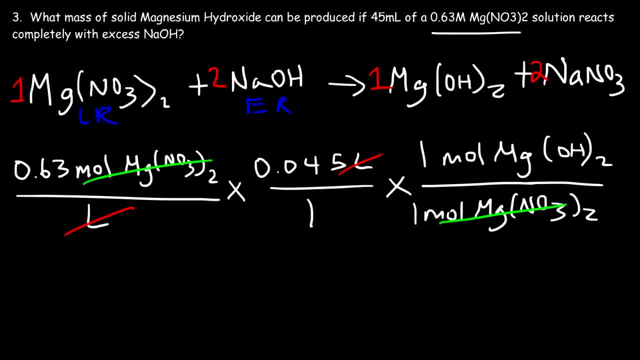 Now the last thing that we need to do is to convert moles into grams, So we need to find the molar mass of magnesium hydroxide. So in that formula we have Mg, two oxygen atoms and two hydrogen atoms. So the atomic mass of Mg is about 24.305 and oxygen is 16.. 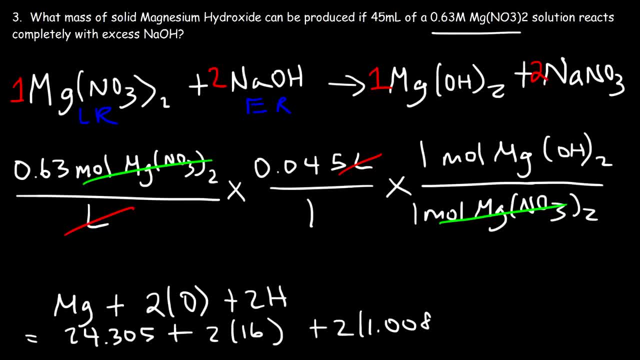 So the atomic mass of Mg is about 24.305 and oxygen is 16.. A Super Rails S chemical hydrogen is 1.008. so if you add up all these numbers you should get 58 point three, two, one grams per mole. so that's the molar mass of magnesium hydroxide. so 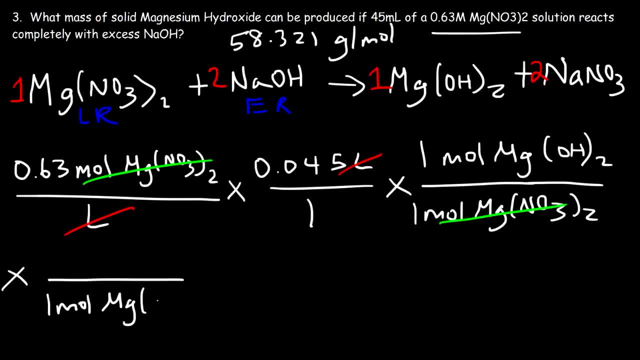 one mole of magnesium hydroxide has a mass of fifty eight, point three, two, one grams. and so now we can get the answer. it's point six, three times point zero, four, five, and then we got to multiply that by fifty eight, point three, two, one, so the mass is one point six, five grams. 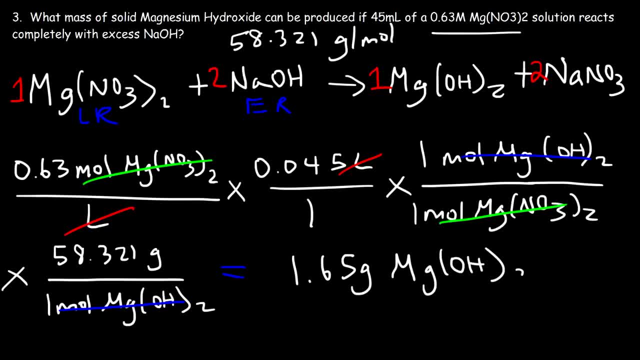 and the mole of magnesium hydroxide has a mass of fifty eight point three, two, one of magnesium hydroxide. So that's the mass that can be produced in this reaction. That's the theoretical yield Number four. what mass of solid calcium? 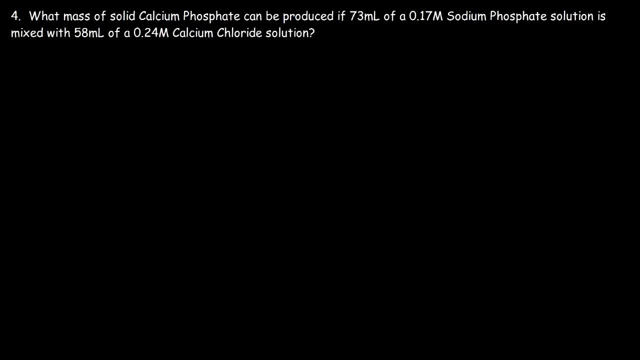 phosphate can be produced if 73 milliliters of a 0.17 molar sodium phosphate solution is mixed with 58 milliliters of a 0.24 molar calcium chloride solution. So in this example we don't know which one is the limiting. 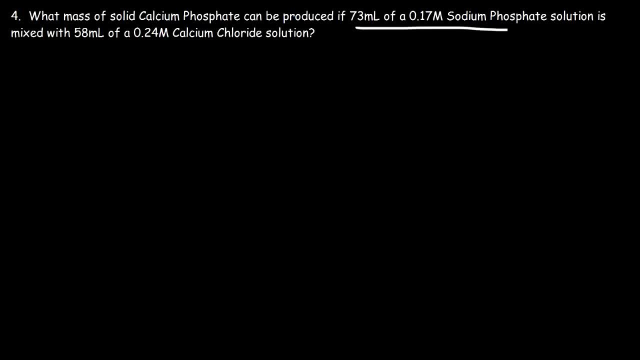 reactant or the excess reactant. We're given the information for both reactants, So, therefore, we need to identify the limiting reactant. What I'm going to do, though, is I'm going to take the information of each reactant and find 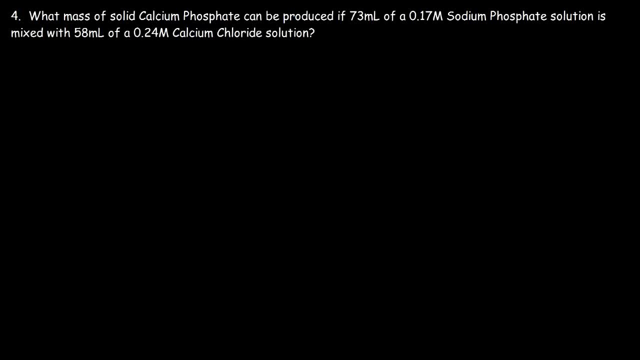 out how many grams of product each reactant can produce. The reactant that produces less product is the limiting reactant, And the quantity of less product will be the actual mass of solid calcium phosphate that will form in this reaction. So we can get the answer and identify the limiting reactant doing it. 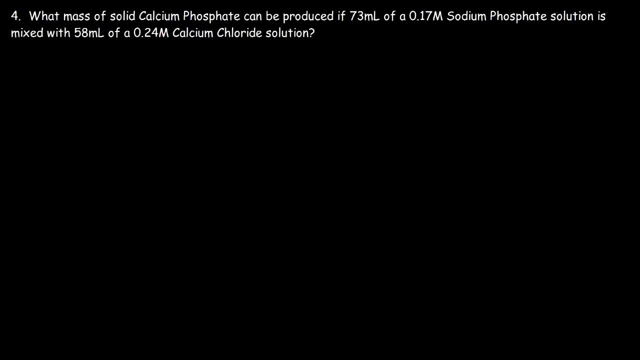 that way. So first we need to write a balanced chemical equation. We're not given a formula of sodium- phosphate, so we need to come up with it ourselves. Sodium has a positive one charge, Phosphate has a minus three charge. So 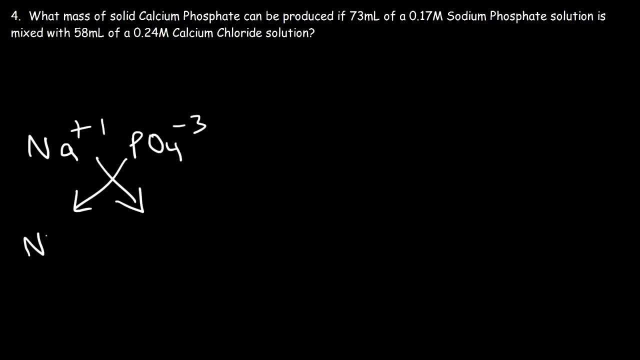 make sure you study the polyatomic ions. So sodium phosphate has a positive one charge. Phosphate has a minus three charge. So make sure you study the polyatomic ions. So sodium phosphate is Na3PO4.. Next we need to write the formula of calcium chloride. Calcium has a positive two charge. 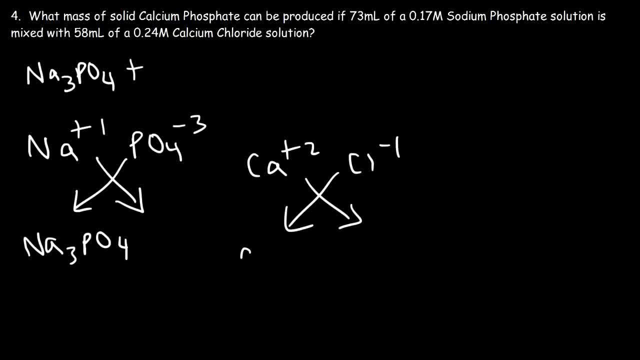 Chloride has a negative one charge, So the chemical formula is Ca1Cl2, or simply CaCl2.. Now sodium is going to pair up with chlorine and they have the same charge, So it's just going to be NaCl. Calcium is going to pair up with phosphate. 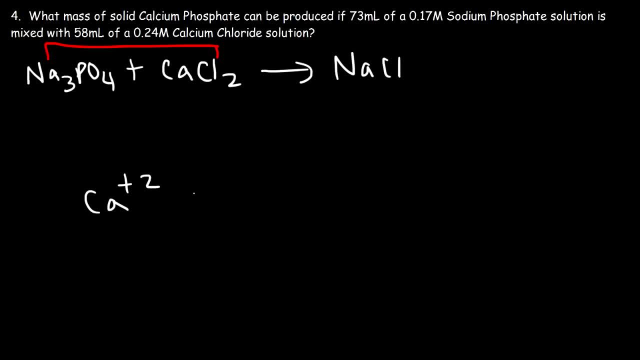 Calcium has a positive two charge, Phosphate has a negative three charge. So they're going to combine in this way. It's going to be Ca3PO4.. So that's the precipitate in this reaction. Next we need to balance the chemical equation. So we have two phosphate ions on. 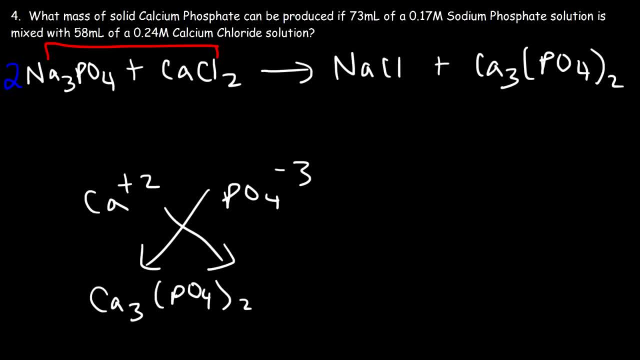 the right side, So we need a two in front of Na3PO4.. And now we have six sodium ions, So we need a six in front of NaCl. And there's six chlorine atoms now, So we need to put a three in front of calcium chloride. 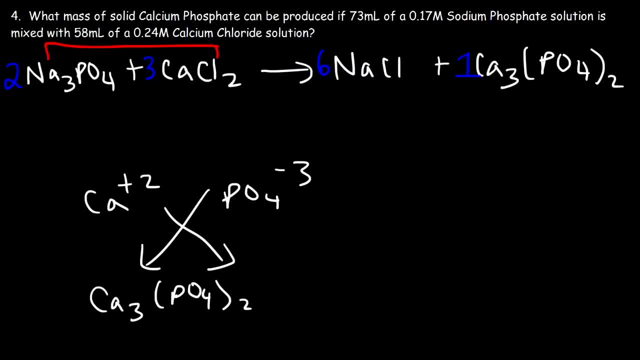 So we need a six in front of NaCl, And there's six chlorine atoms now, So we need to put a three in front of calcium chloride, And now everything is balanced. Now let's start with sodium phosphate. Let's see how many grams of calcium phosphate can be produced if all of the 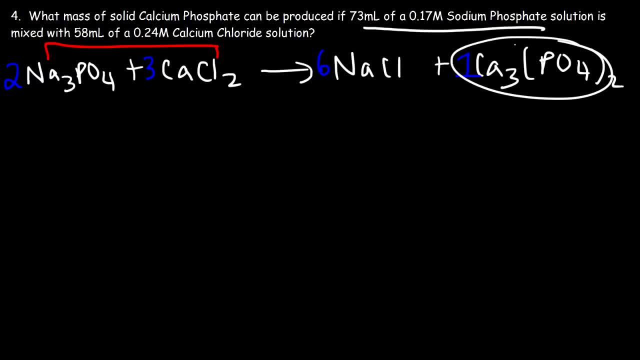 sodium phosphate reacts in this chemical reaction. So this problem is going to be similar to number three, but we're just going to follow that same process with each reactor. So I'm going to start with 0.17m. So there's 0.17 moles of. 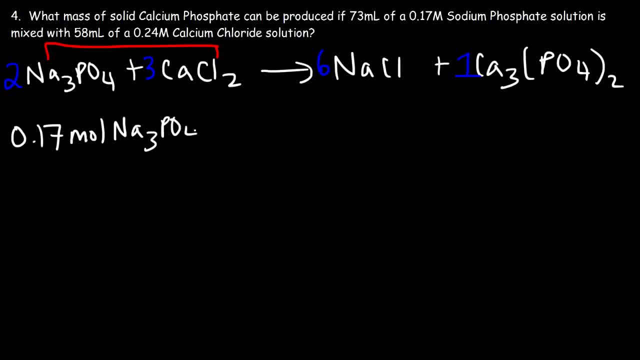 sodium phosphate per liter of solution. And next let's multiply by the volume in liters: 73 milliliters is the same as 0.073 liters. Now let's convert sodium phosphate into the product calcium phosphate. The molar ratio is 2 to 1.. So we're going to put two moles of Na3PO4 on the bottom. so 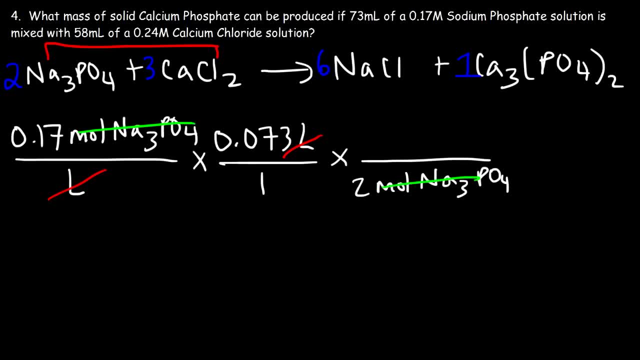 that these two units will cancel And we're going to put one mole of calcium phosphate on top. Now the next thing that we need is the molar mass of calcium phosphate, So there's going to be three calcium atoms in that compound, two phosphorus atoms and 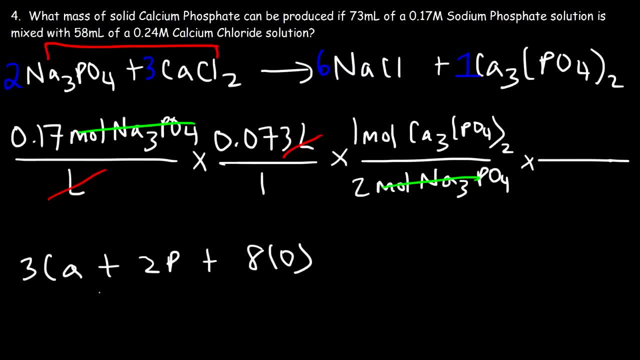 four times two is eight, so eight oxygen atoms. The atomic mass of calcium is about 40.08.. Phosphorus is 30.97.. And Oxygen is 16.. So the molar mass is 310.18 grams per mole. So one mole of calcium phosphate has a 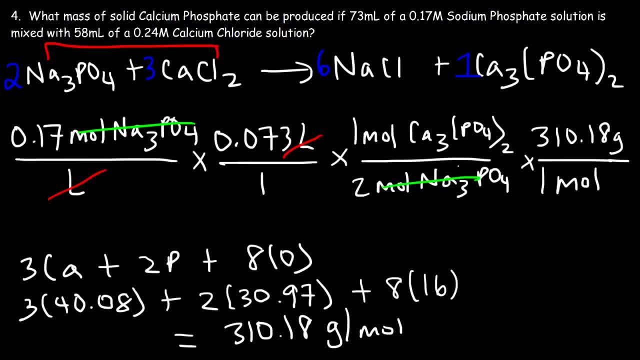 mass of 310.18 grams. So now let's get the answer: 0.17 times 0.073, divided by 2 times 310.18.. So the mass produced is going to be 1.925 grams of calcium phosphate. So I'm going to. 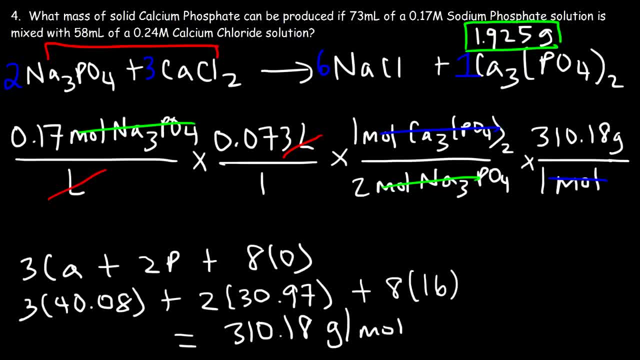 highlight that in green, And I'm going to highlight this in green So just to keep track that this mass came from this reactant. It's based on sodium phosphate. Now let's follow the same procedure, but with calcium chloride. So let's start. 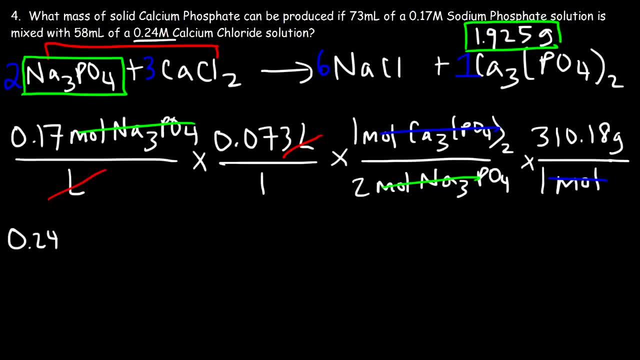 with the molarity of calcium chloride. So it's 0.24 moles per liter, And now let's multiply it by the volume, which is going to be 0.058 liters. Now the molar ratio between calcium chloride and calcium phosphate is 3 to 1.. 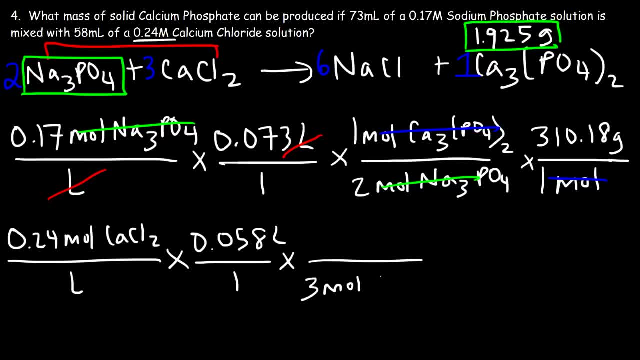 So we're going to have three moles of calcium chloride on the bottom and one mole of calcium phosphate on top. Now the last part is going to be the same. The molar mass of calcium phosphate is not going to change. It's going to stay 310.18 grams per mole.